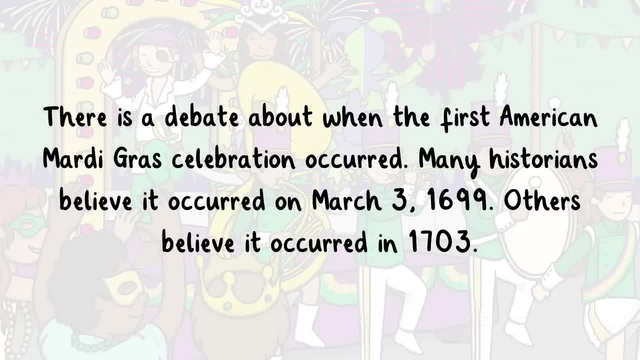 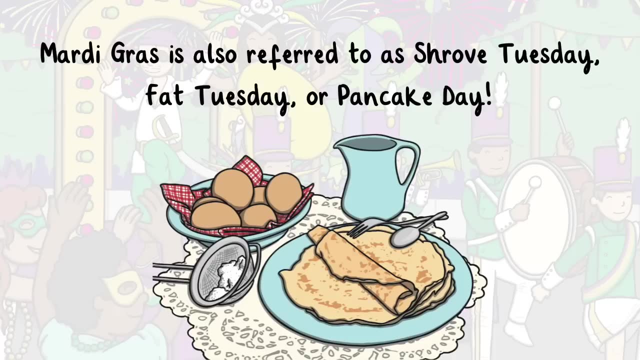 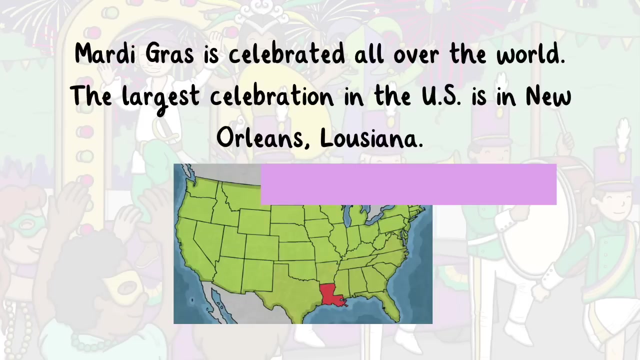 Many historians believed it occurred on March 3rd 1699. Others believe it occurred in 1703. Number three: Mardi Gras is also referred to as Shrove Tuesday, Fat Tuesday or Pancake Day. Number four: Mardi Gras is celebrated all over the world. The largest celebration in the United States is in New Orleans, Louisiana. 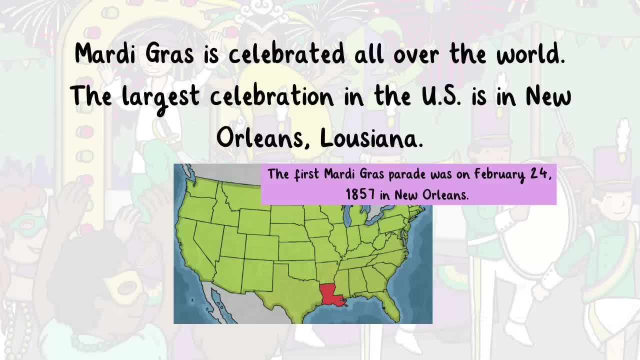 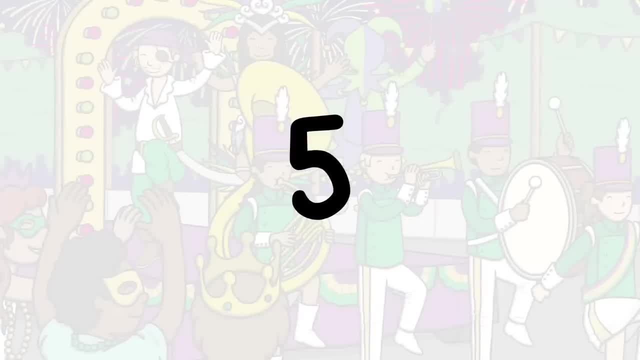 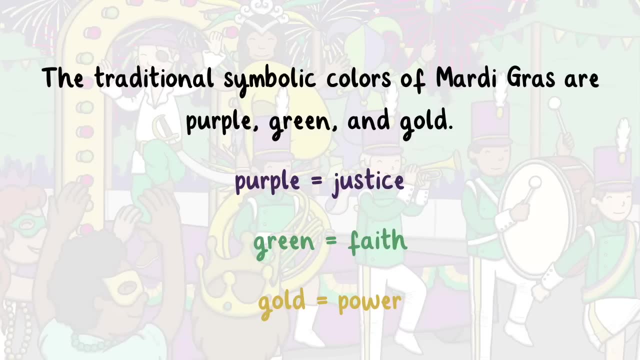 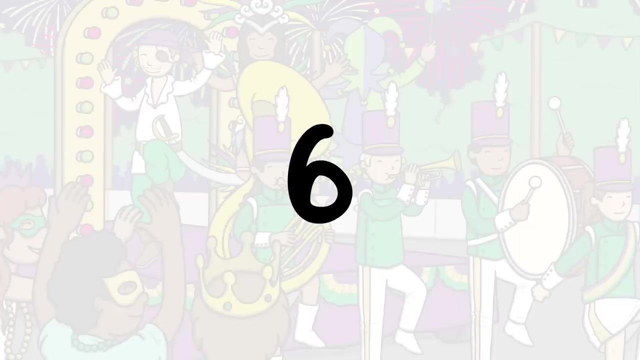 The first Mardi Gras parade was on February 24th 1857 in New Orleans. Number five: The traditional symbolic colors of Mardi Gras are purple, green and gold. purple symbolizes justice, Green symbolizes faith and gold symbolizes power. Number six: Crews are an important part of Mardi Gras. 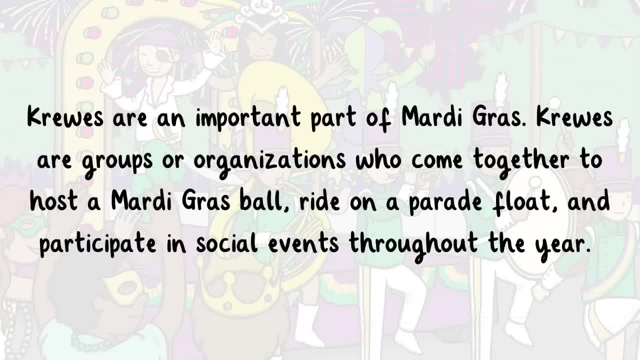 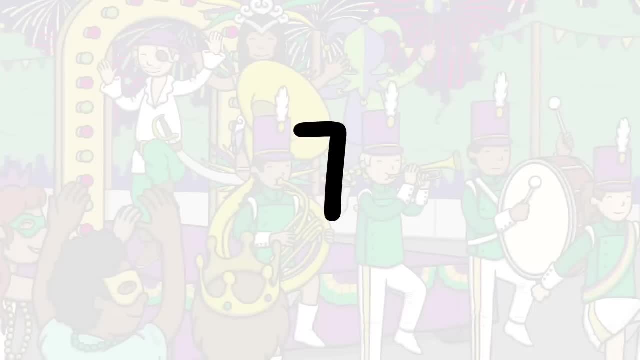 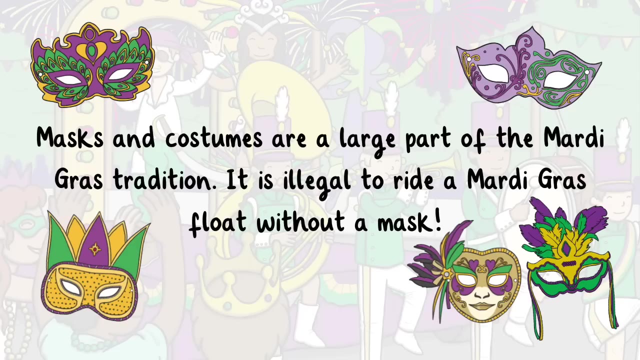 Crews are groups or organizations who come together to host a Mardi Gras ball, Ride on a parade float and participate in social events throughout the year. Number seven: Masks and costumes are a large part of the Mardi Gras tradition. It's illegal to ride a Mardi Gras float without a mask. 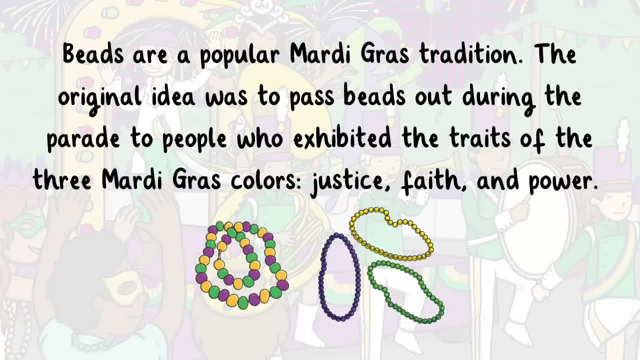 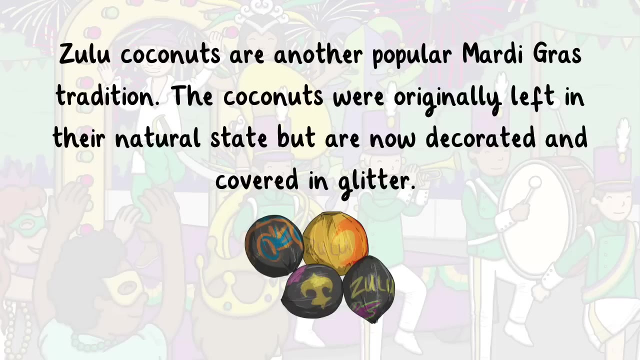 Number eight: Beads are a popular Mardi Gras tradition. The original idea was to pass beads out during the parade to people who exhibited the traits of the three Mardi Gras colors: justice, faith and power. Number nine: Zulu coconuts are another popular Mardi Gras tradition. 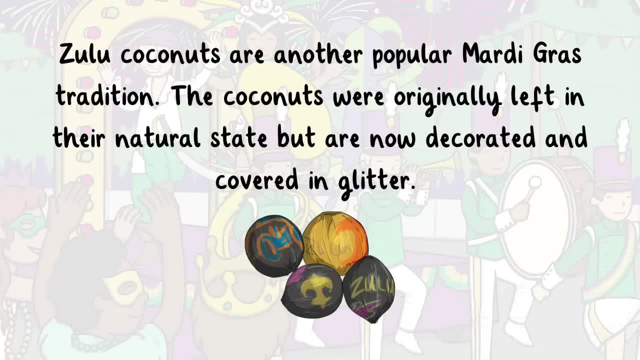 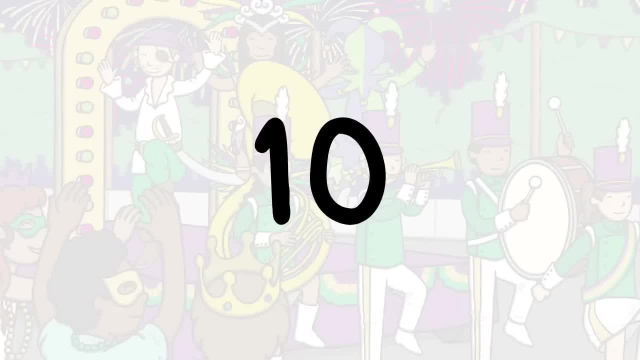 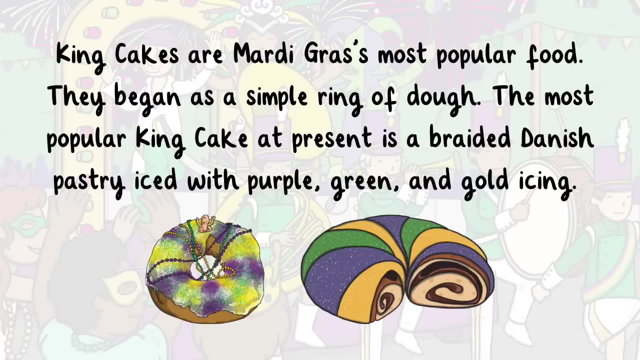 The coconuts were originally left in their natural state but are now decorated and covered in glitter. Number ten King cakes are Mardi Gras' most popular food. They began as a simple ring of dough. The most popular king cake at present is a braided Danish pastry iced with purple green.